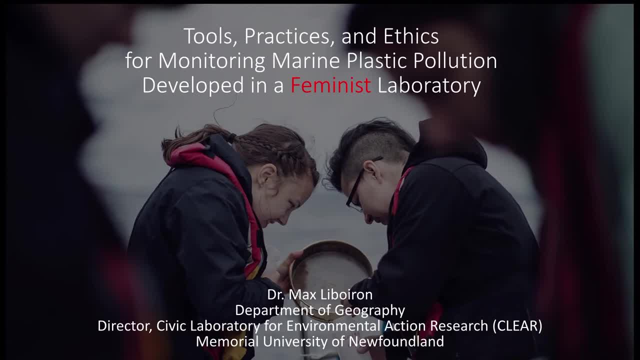 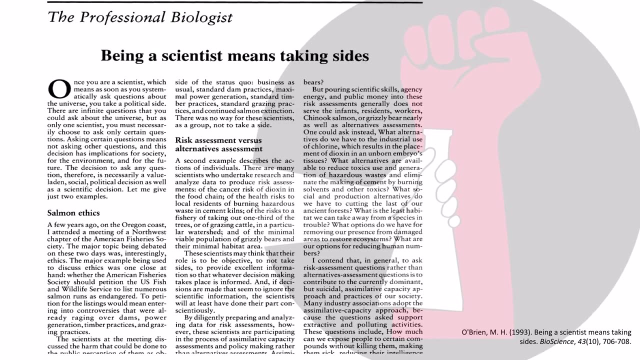 But in each case we're going to talk about how our practices come out of a commitment to community concerns, feminist ethics and collaboration between scientists and non-scientists. This is what makes our science fairly unique as a feminist laboratory. So sometimes when people find out that I'm a feminist scientist and run my laboratory as a feminist lab, they say: well, does that mean you're biased? 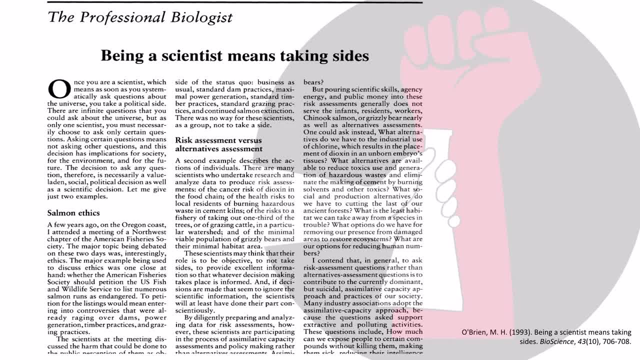 But for a long time we've known that being a scientist means taking sides. This is an excellent article from 1993, Mary O'Brien, who says: as soon as you pick a research question, that's a political decision. So if you decide, for example, to research how healthy salmon can be in a particular stream, 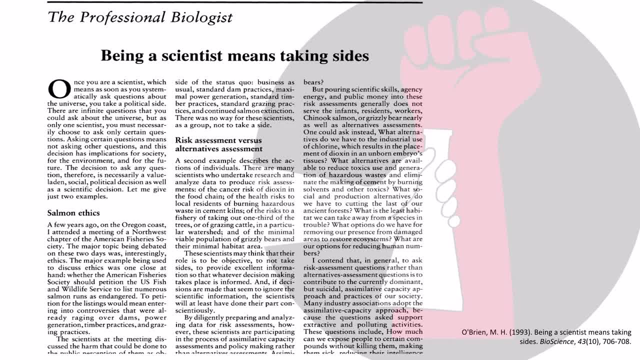 to try and stabilize their population. that's a very different thing than if you are trying to research how to best pressurize water to get it into some shale, to force gas bubbles out which is fracking. As soon as you've chosen one of those two things, you've aligned yourself with different industries, with different politics, with different funding institutions. 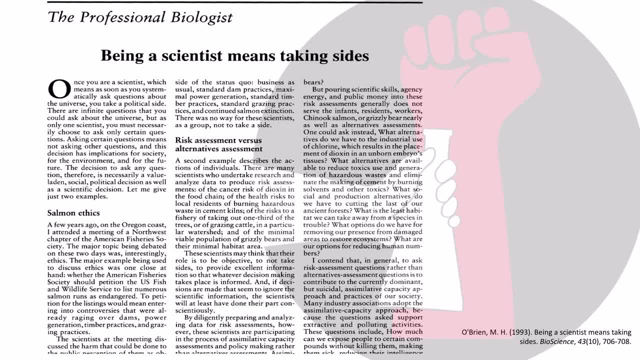 and you've already made political decisions, even if you don't mean to. This also includes who you choose to work with, who you choose to collaborate with or not. All of these have ramifications in the social and cultural worlds. They're all part of science, not separate from it. 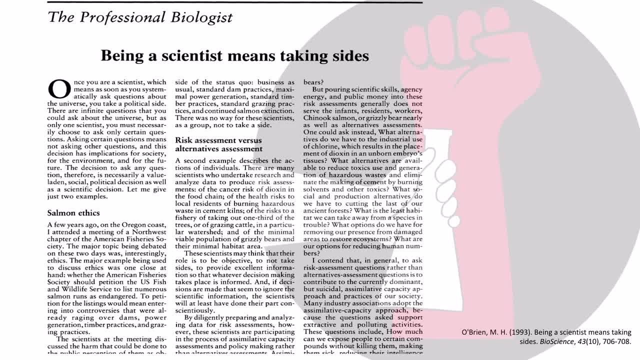 And so feminist science says: by owning this, by being very clear about it, you actually improve your objectivity. It's called strong objectivity. So I'm going to give you a quick introduction to feminism. So feminism is a social movement and there are lots of different types of feminism. 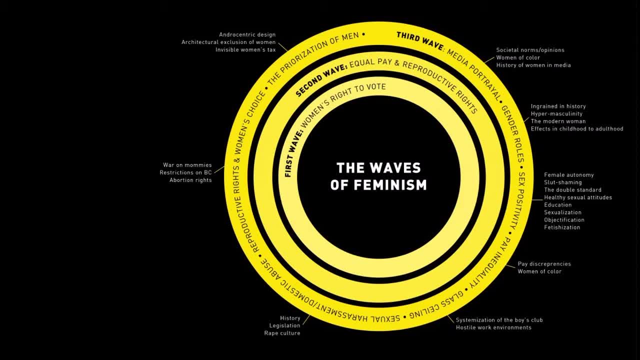 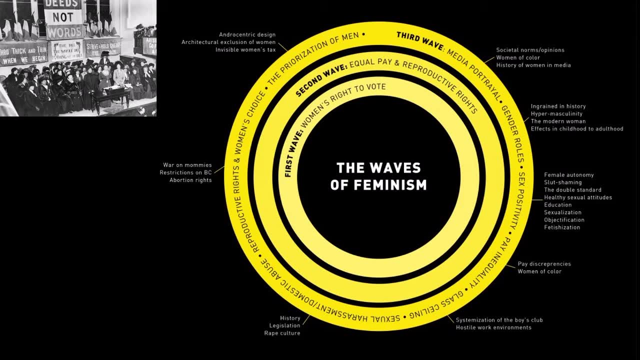 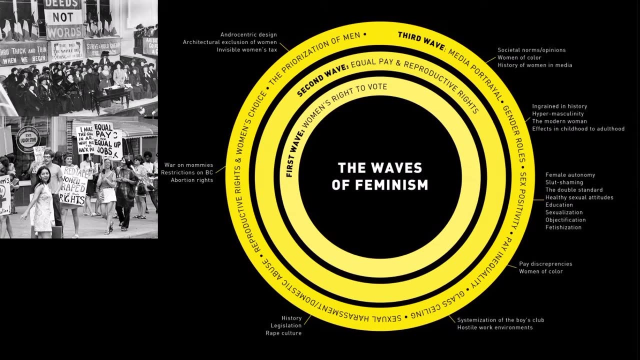 One of the ways you can describe the different kinds is through waves, historical waves. So the first wave of feminism is the suffragettes fighting for the right to vote, to be the same type of citizen as men. The second wave of feminism coincides with the United States civil rights movement. 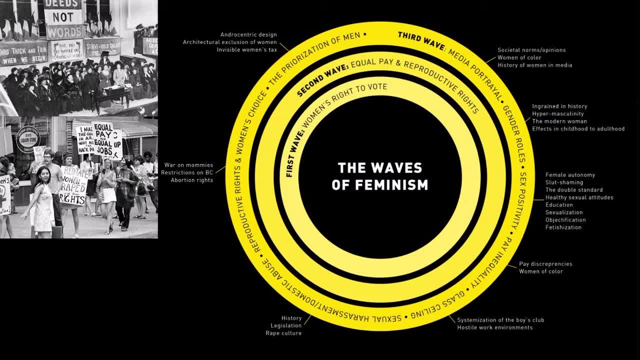 And it said: well, even though we have the right to vote like men, we're still not, in our daily lives, equal. We don't get equal pay for equal work. We don't have reproductive rights or the rights to our own body. 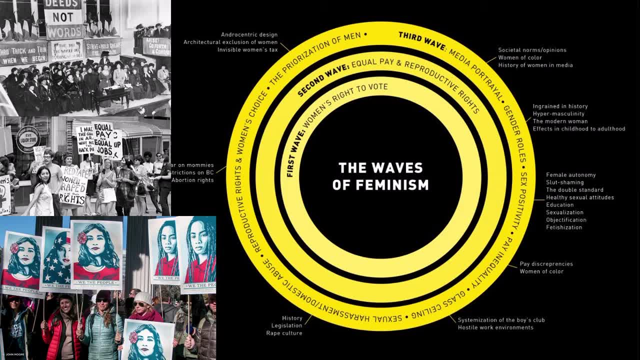 And then third wave, feminism, which is, some people say what we're in right now, although the other two feminisms are still at play. I like to think started when someone looked around and said, wow, this is a really white movement, And it turns out you're not never just a woman. 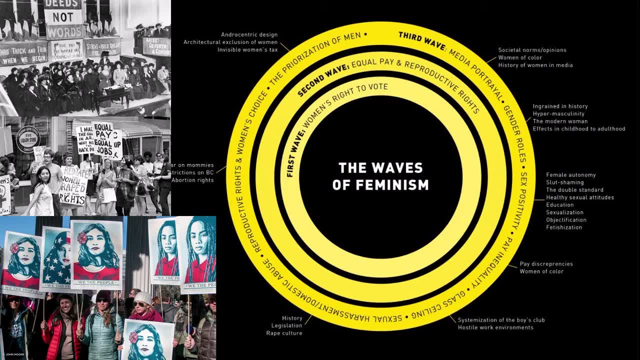 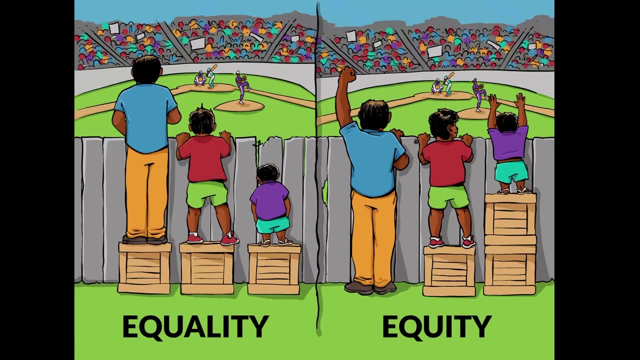 You are also of color or white, You're also above or below the poverty line, You're also abled or disabled, You're also immigrants or not, And so third wave feminism is characterized by looking at these different, intersecting things. Third wave feminism is characterized by a move from equality- where you treat everyone the same- to equity. 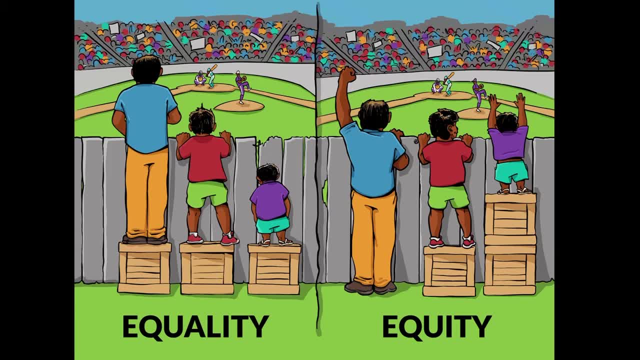 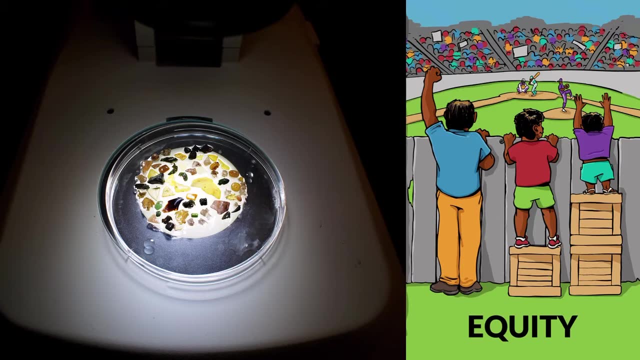 where you recognize that people start from very different locations And so treating them exactly the same might actually not address those different locations. So what does that look like in science? Well, in science, let's say that you want to monitor environmental plastics. 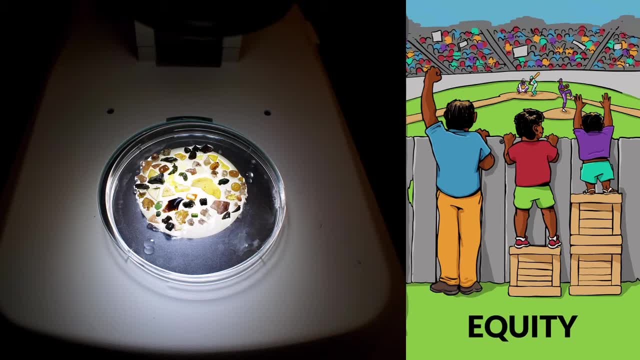 And so you give three people citizen science methods, Right? So, even though they're not scientists, you give them sensors for looking for marine plastics. But one of them lives in Labrador, the northern part of this province, And the electricity doesn't always work there. 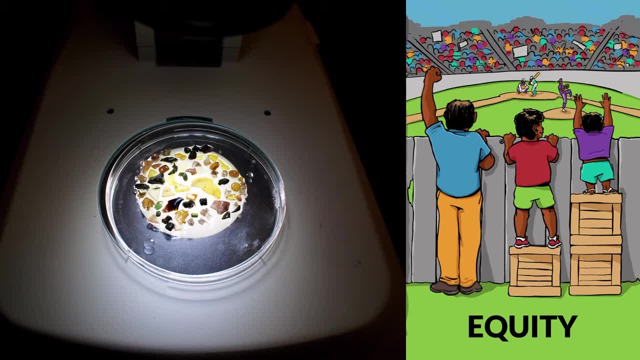 And so if they have a digital readout on their device, they can't actually use it. Another person works two jobs and is in debt and so doesn't have time to use it. And the third person you give it to has a degree from Oxford and a really sexy accent. 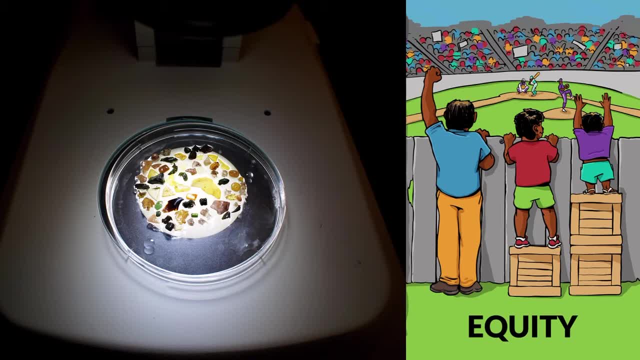 And everyone believes what they say. So even though you've treated them exactly the same under an equality model, you haven't actually changed how science get done. You can't even get some of the science done because people start from different social locations. So this is a very simple way of looking how you can bring equity into science. 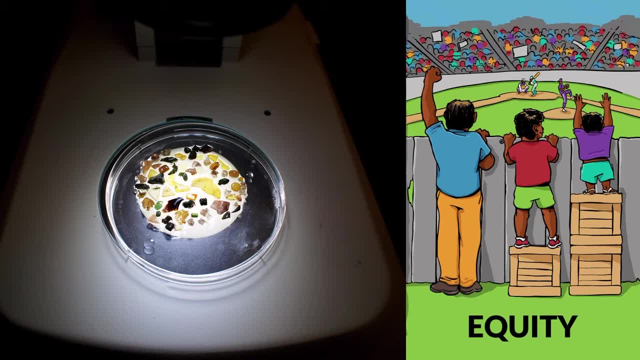 I'm going to give you a quick lesson on marine plastic pollution, a quick introduction, And then I'm going to get to how we try and put equity into every aspect of our research on marine plastic pollution in Civic Laboratory. So you probably know that there are plastics in every ocean in the world. 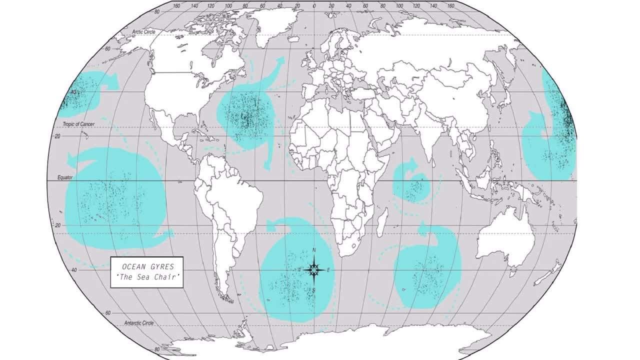 They tend to accumulate in these places called gyres, These giant ocean currents that swirl around that have plastics in the middle of them. Last summer, I was fortunate enough to be able to travel through the North Atlantic Gyre, which is the one closest to Newfoundland. 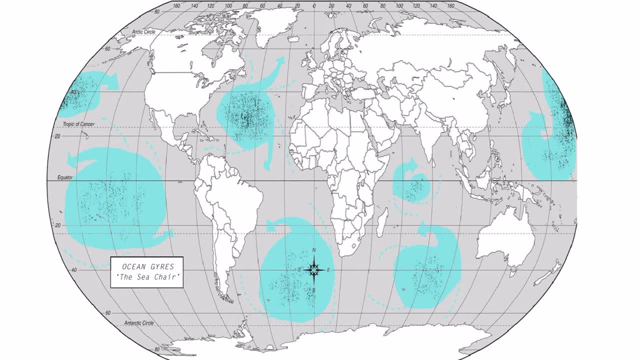 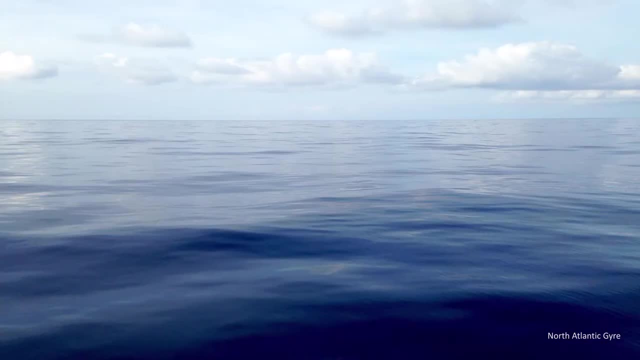 And as our devices started pulling up more and more plastics, which signaled that we were in the middle of the gyre, I leaned over the side of the boat and I took a photograph so you could see what it looked like: Pretty calm, Not a lot of plastics floating here. 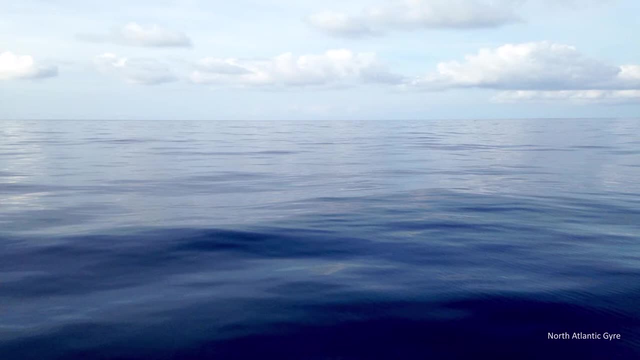 And that's because people often imagine that marine plastics are just plastics that you know in everyday life- bags and bottles just located in the water. But in fact marine plastics are very different than land plastics. Over 90%- nearly all- marine plastics are smaller than a grain of rice. Less than five millimeters. They're called microplastics. There's a bunch of different problems associated with plastics of different size, So bigger plastics can entangle animals right- Ghost fishing nets that aren't attached to fishing boats anymore, for example. 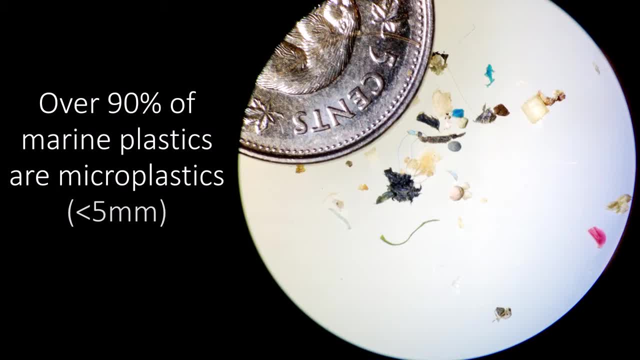 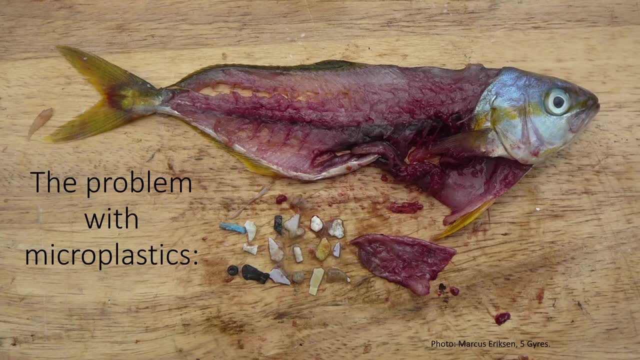 But the problem that we concentrate on? the problem that we focus on is ingestion. Because plastics are so small, they fragment from larger pieces into smaller pieces. Although some start that small, like in face scrubs, Because they're so small they can be ingested by a wide range of animals. 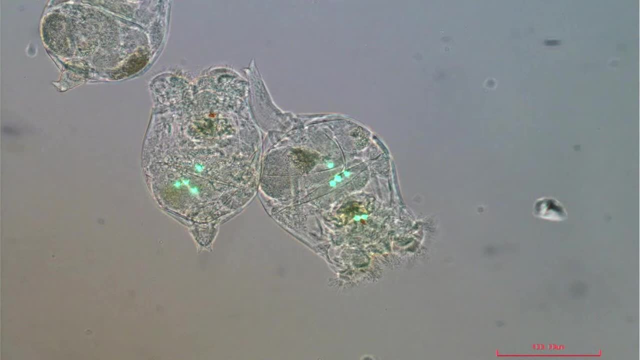 This is a photograph we took in the lab last week. These are plankton- rotifer plankton- with tiny little microbeads in them- Plastic beads from face wash. Now, just because an animal eats plastic doesn't mean they're automatically harmed. 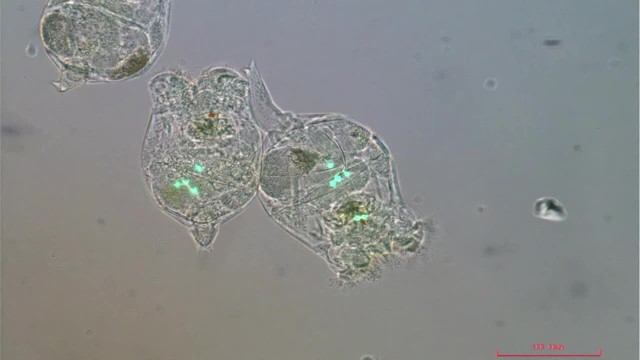 So you might have seen the Chris Jordan photographs of albatross with plastics in their belly as they decay. Those birds did not die from plastics. Certainly not necessarily, And you know this- because of dogs. So say you have a dog, I have a dog. 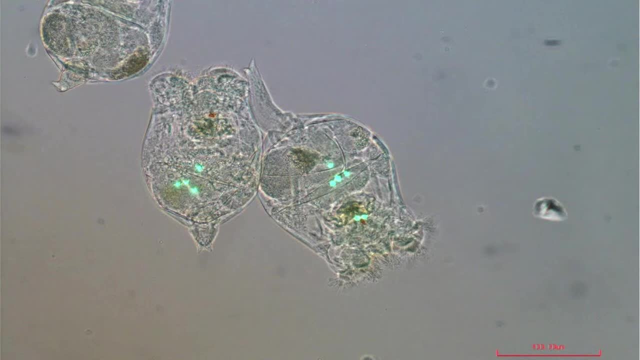 He eats plastic almost every day. He eats a lot of non-food items, But he's alive. Most dogs are alive. There's not a species problem with dogs, And that's because just because you eat plastics or non-food items doesn't mean that you're harmed automatically. 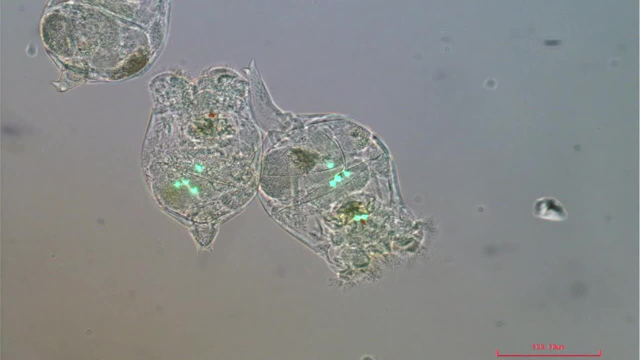 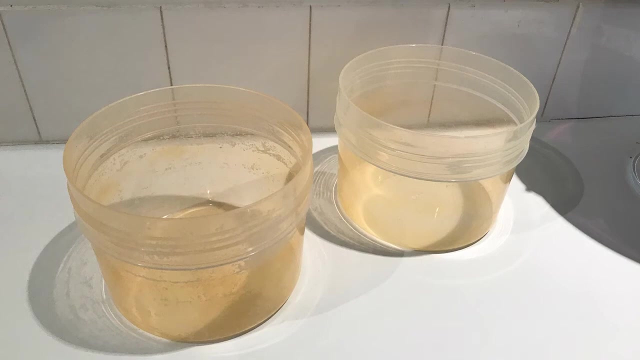 In fact it's quite rare. We don't see it very often in science. What we're concerned about is how plastics absorb oily or hydrophobic chemicals. So if you've ever had curry or spaghetti and you've put it in Tupperware and then you can't scrub the orange color out of the Tupperware, 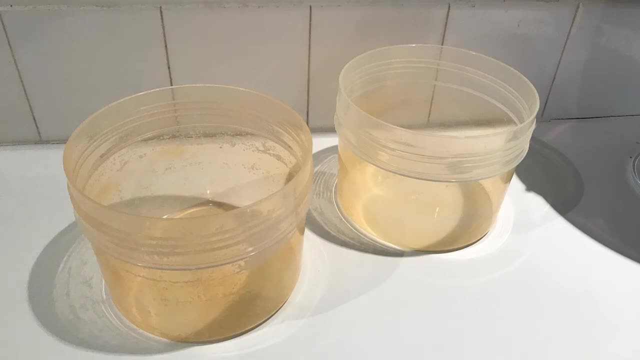 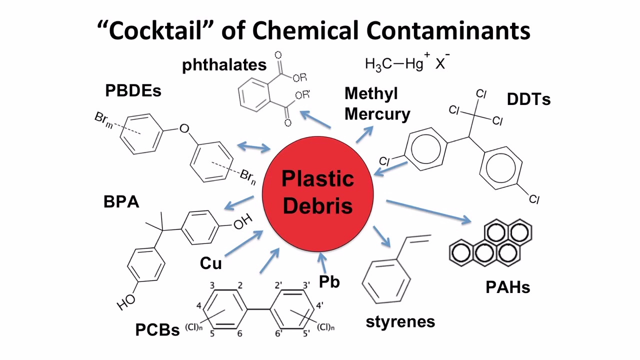 that's a manifestation of how plastics absorb oily chemicals, like spaghetti sauce in this case, And what happens in the hot, abrasive, acidic conditions of a stomach is those chemicals will move out of the plastic and into the animal's tissue. The chemicals that tend to be absorbed by plastics include the chemicals that are already there, like BPA or phthalate. 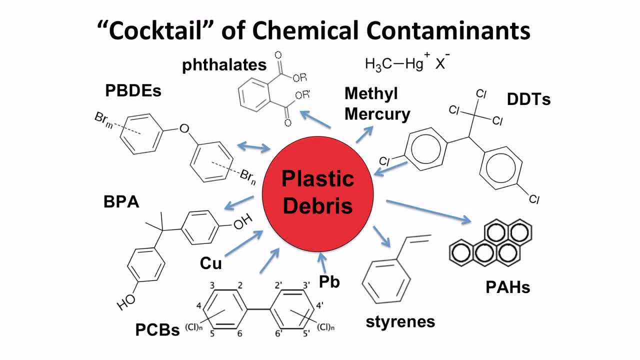 But also flame retardants, pesticides, heavy metals, As plastics move from land into the ocean. about 80% of plastics are from land. They move through parking lots, through sewage systems, out through bays and into the water, And they can absorb up to a million times more chemicals than the surrounding water. 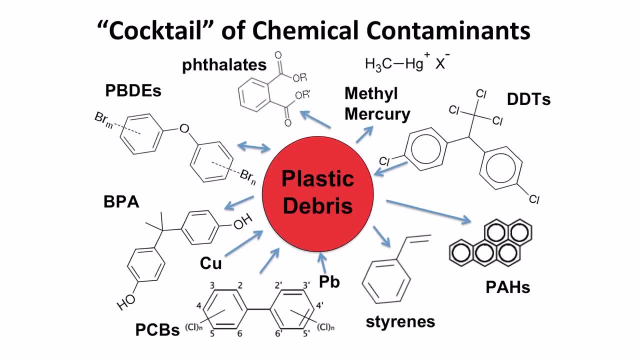 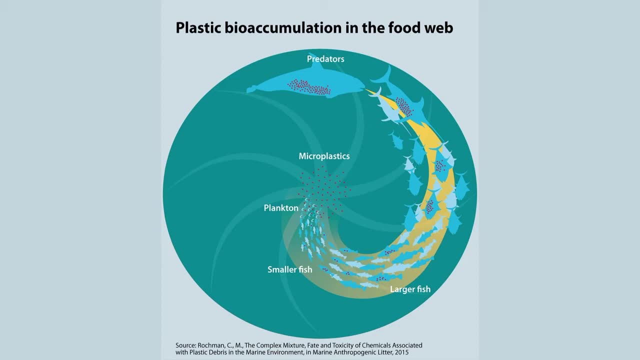 We actually nicknamed them poison pills because they attract all these different chemicals. Now when an animal eats these, the chemicals can be absorbed into their tissue. Those chemicals can also biomagnetize. They can modify up the food chain, so smaller animals will have a little bit of plastics and their chemicals in them. 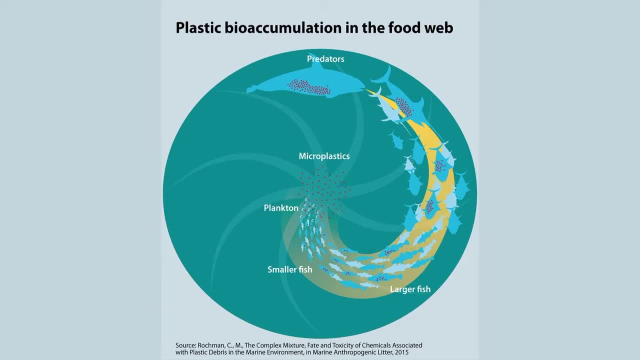 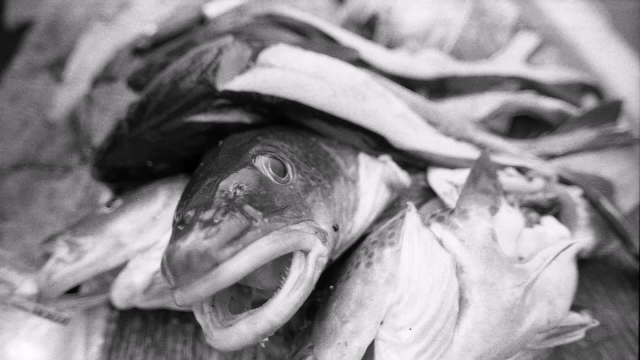 but predators will have more, including humans. This is a big concern in Newfoundland because Newfoundland depends on fish Culturally, for livelihoods, for sustenance. Newfoundlanders eat a lot of fish And particularly people who are rural, who live below the poverty line. 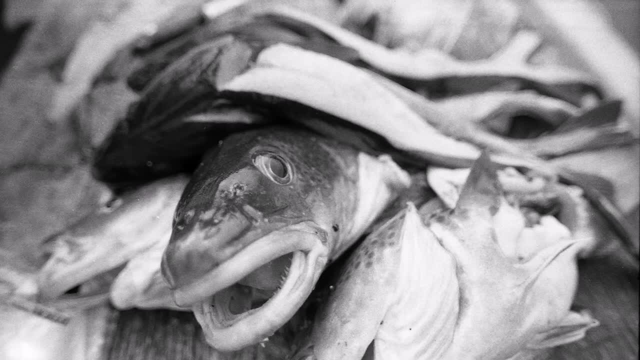 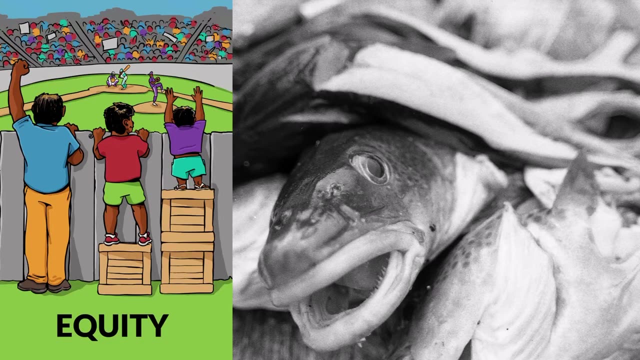 and people who are in Labrador, the sub-Arctic region of the province, who are mostly indigenous. So what this means is that you have an equity issue in our research question. This is why, as a feminist laboratory, we research marine plastics. 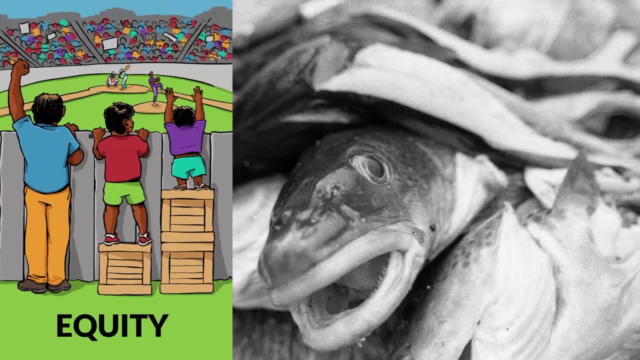 Just because you're poor, rural or northern or indigenous, you end up at greater risk of the problems associated with marine plastics. So the way we've chosen our research question, the thing that we research, aligns with these people who are at higher risk of harm. 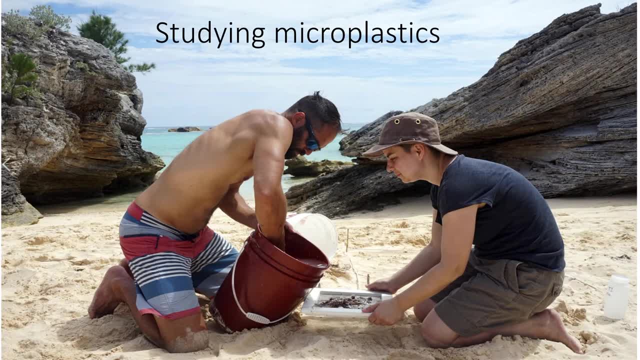 So how do you study marine plastics? Well, there's this method that is being shown in this photograph in Bermuda. The United Nations, the United States, NOAA and the European Union have all agreed that there's a basic universal protocol that you use. 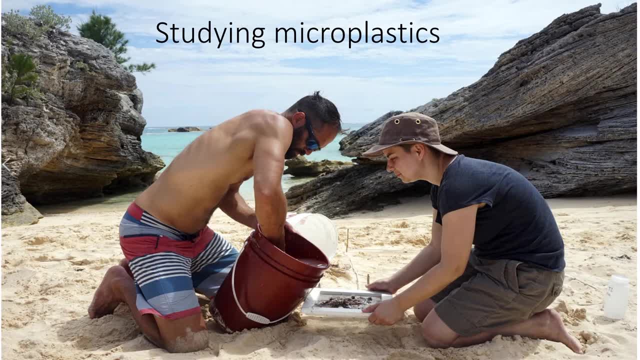 when you're looking at shoreline plastics. That's what we're doing here. You basically put a square in the sand called a quadrat. You scoop all the sand out, You put it in a bucket, swish the bucket around, The plastics float to the top. 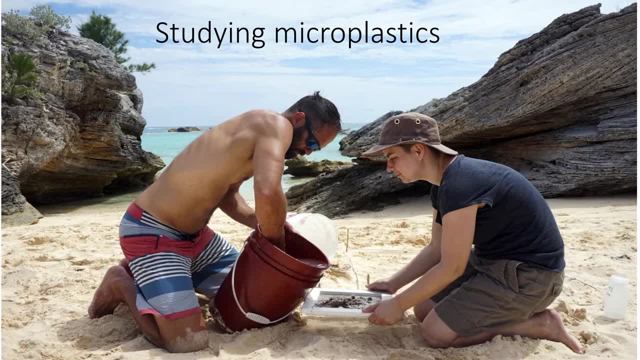 You pour them out and you can then see the densities, numbers, types etc. of plastics in an area. This is again a universal protocol so that people in different parts of the world can compare across a global problem. This is Newfoundland. 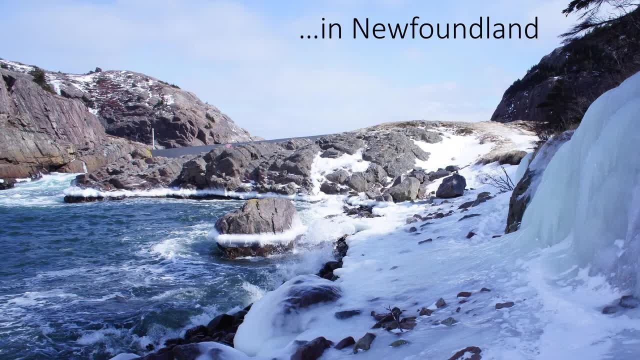 I dare you to sieve that beach. There's no sand. There's very little sand in Newfoundland or really the subarctic or arctic regions. It tends to be rock, ice and mud. And what we found over and over again, no matter what sort of protocol we're looking at, 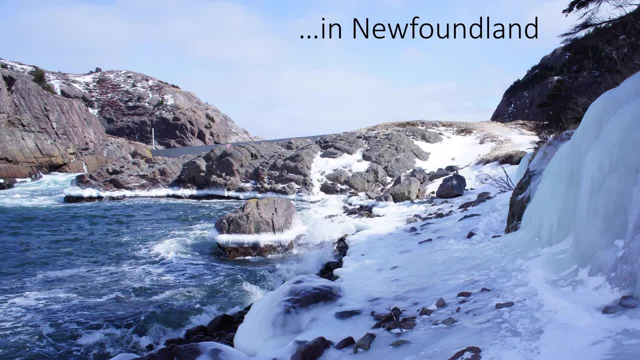 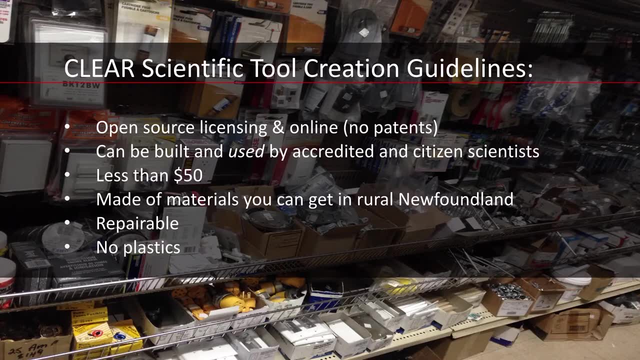 very few of them work in those conditions, in these extreme northern environments, So we end up having to make a lot of our own scientific tools. The way we make scientific tools is again based on equity, this idea that it shouldn't just be us with our big grants and the big university doing the science, but that people 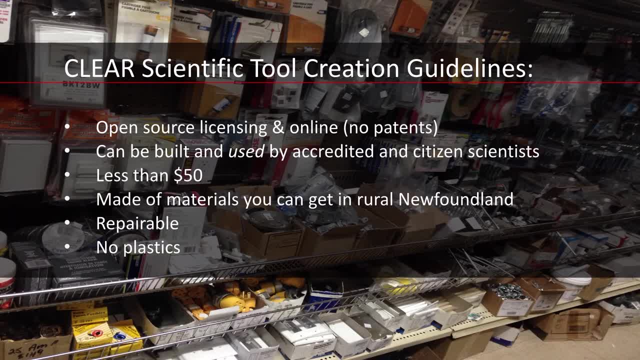 who live in rural places, people who eat a lot of fish, people who depend on the land, should also be able to answer their own research questions. So when we're building our scientific tools, we have a few guidelines. First of all, they have to be open source and online. 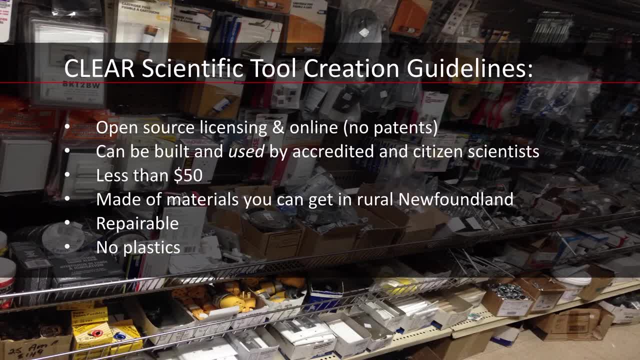 We don't patent them or privatize them. Everyone needs to be able to access them. They should be able to be built and used by people with and without science degrees. So they can be complex, but they can't be overly complicated, And this is specifically for our instructions for how to build them. 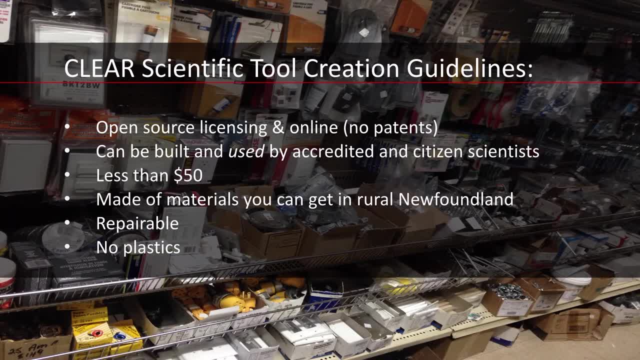 They should cost less than $50.. Now your average rural Newfoundlander is not going to spend $50 on research, but a group of Newfoundlanders who live in an area might, or community groups. Now you have to be able to actually make it in rural Newfoundland. 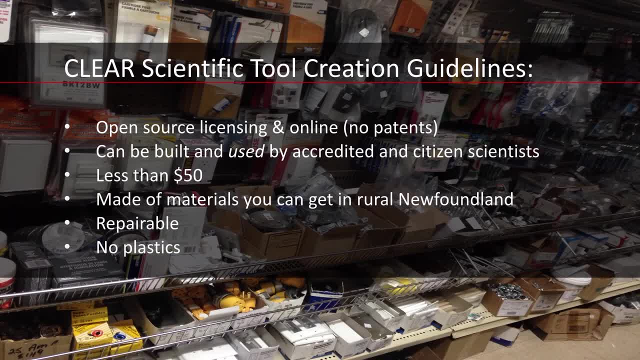 So most rural Newfoundland communities either don't have a store or only have one or two stores. So the photograph in the back of this is actually of the general store on Fogo Island in a place called Joe Bat's Arm. We went around and we photographed everything in the store. 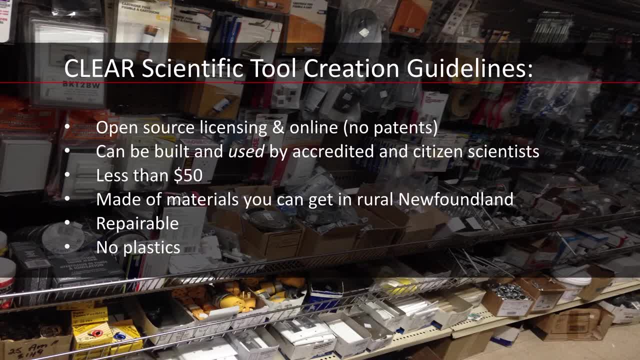 and then, when we build things, we can only use the materials in those photographs. People have to be able to repair, hack, change and augment to fit their areas, their areas of research. And how about if we don't make our devices out of plastic? 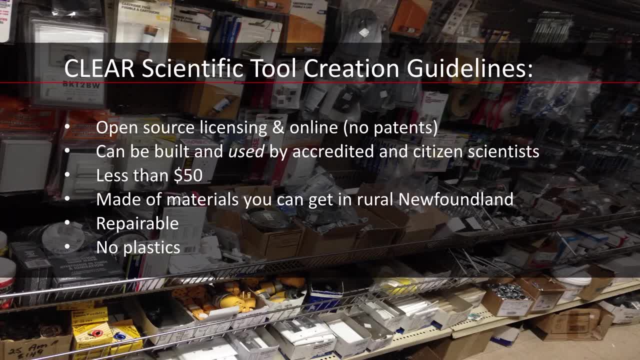 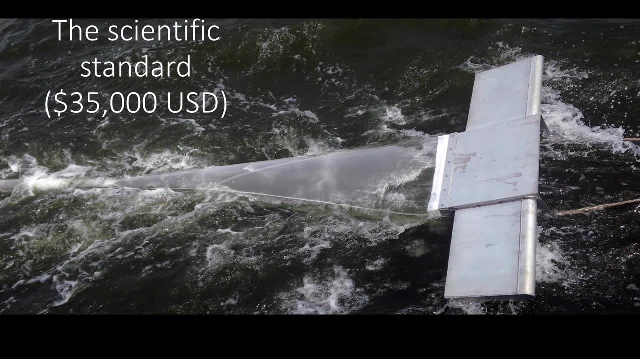 and potentially contribute to the problem we're trying to solve. So what do our instruments look like? They don't look like this. This is the scientific standard. It's called the mantitrall. It's built like a manta ray. 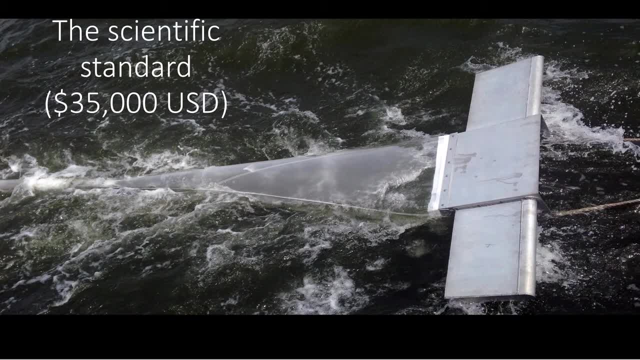 Basically it's a very expensive butterfly net. Water moves through the mantitrall. All the floating things, including plastics, gather in that net in the back and that is a sample. It costs $3,500 US dollars. Only a few places create it and it's really quite heavy. 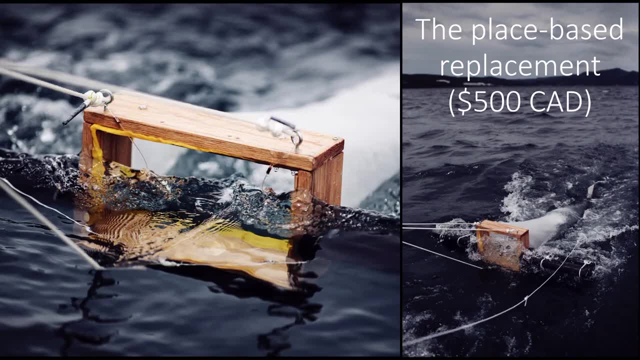 Too heavy for, say, a fishing vessel. What we've designed is the ladytrawl. So there's the mantitrall and the ladytrawl. Lady stands for low-tech aquatic debris instrument. It was co-designed with my students and it's built with things you can get in Newfoundland. 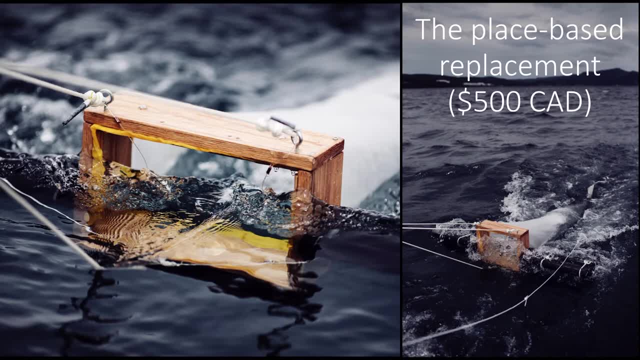 so wood, raincoats, piping, And it only costs $500 Canadian dollars. Almost all of that is for the net in the back, which you can order online. It is the exact same as the mantitrall. Now the ladytrawl gathers the exact same data as the mantitrall. 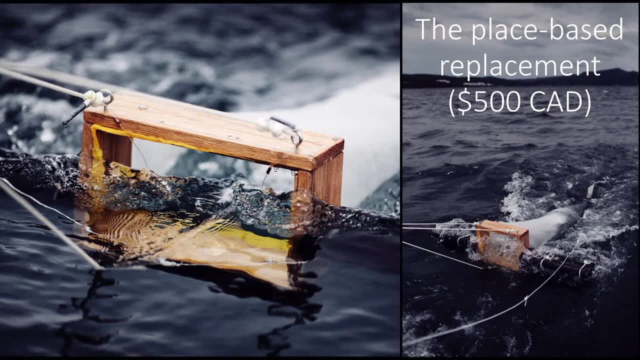 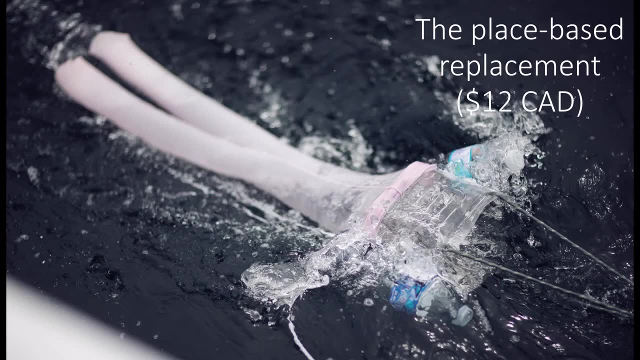 So it's scientifically sound. We validated it. But $500 is still pretty cheap and doesn't meet our guidelines. So this is babylegs. Babylegs is called babylegs because she's made of baby tights. It turns out you can get baby tights in most rural Newfoundland communities. 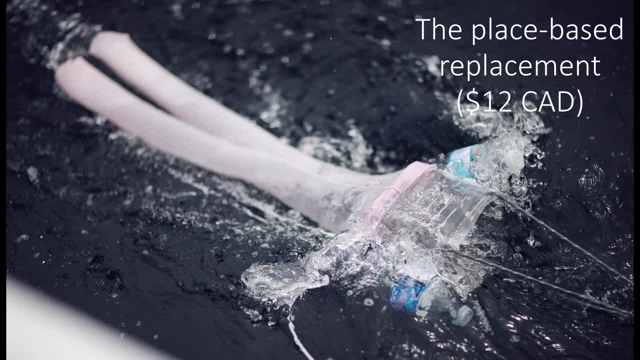 because there are a lot of Christians there and if you're going to baptize your baby, the baby's got to be wearing tights. This is something I've learned, So this is a pair of baby tights using a plumber's clamp. 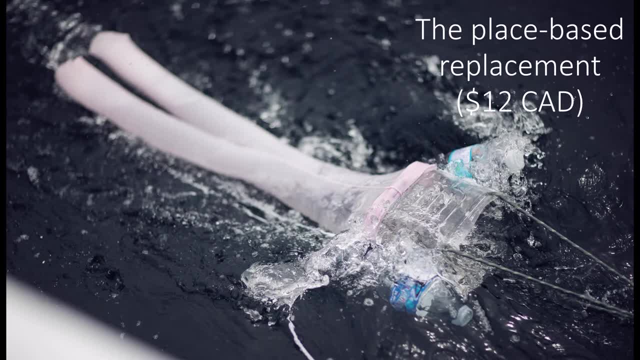 to stick it around a container and then dragged through the water: $12.. Easy to make, Easy to get the stuff for, Easy to hack, Easy to change. Also made of plastic. So the guidelines that we have about how to build them. 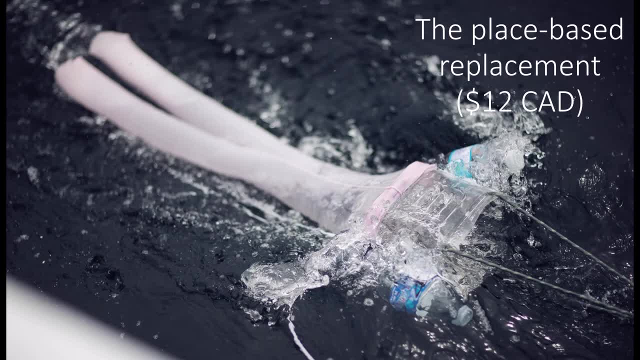 we always think about how can we meet economic, environmental and social justice whenever we do this. So in this case it turns out that if you want to make something cheap and accessible, you can't not make it of plastics because oil is so subsidized. 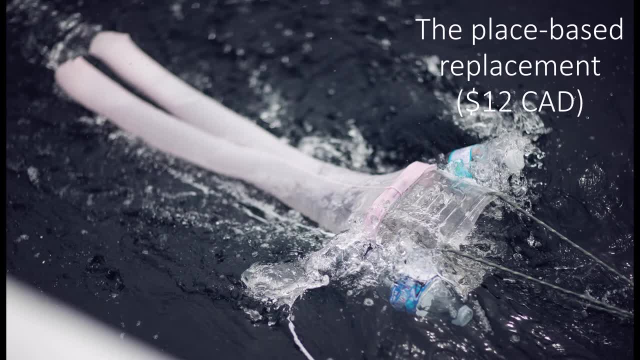 especially in Newfoundland. So this is the sort of compromise we make. We use equity and access as guiding principles. We think about what someone in rural Newfoundland requires and then we build it to those specifications. Now, tools aren't the only thing we build and make public. 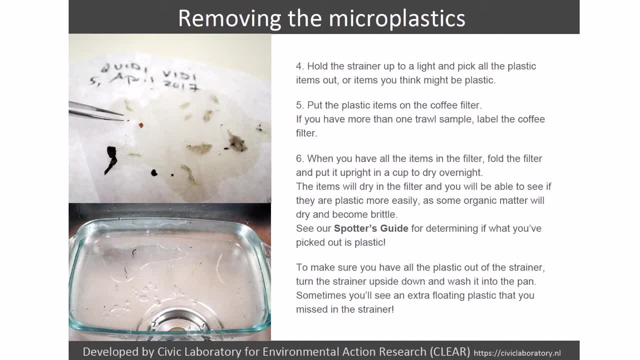 Our protocols. that is how we do the research. how you analyze the plastics are also public. So this is from a how-to guide for how to analyze plastics from trawls. In the top picture there's a coffee filter. You can also use a fancy silo. 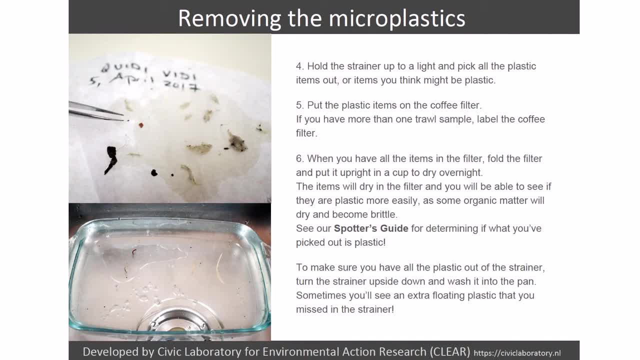 It's a scientific filter, but they do the same job. We use Pyrex casserole dishes, So I want to emphasize that, because humility and solidarity are a major part of our science, meaning that if we take people who don't have science degrees seriously as people who have research questions, 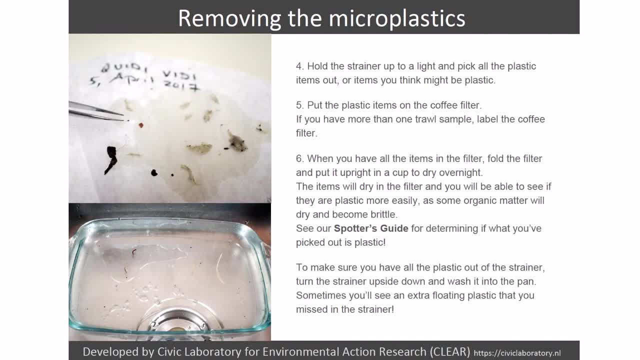 research needs and then try and provide the infrastructure for that. we don't then save the cool, good, expensive equipment for ourselves. We use the exact same tools that we make, build and offer to non-scientists. This is really important to our work and is a main part of our ethics. 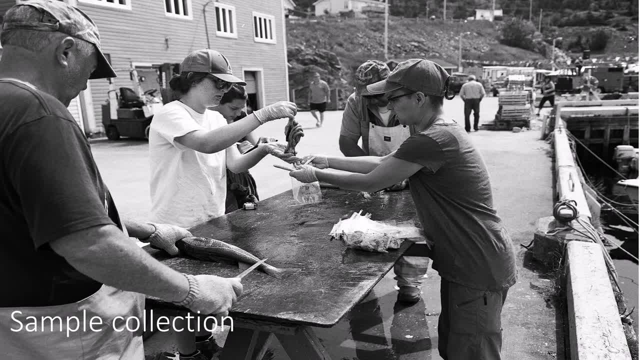 The last thing I'm going to talk about is our sample collection for ingestion. So every summer everyone in Newfoundland, for two to four weeks, can go out and catch as many fish as they want. Well, that's not true. Five per boat per day. 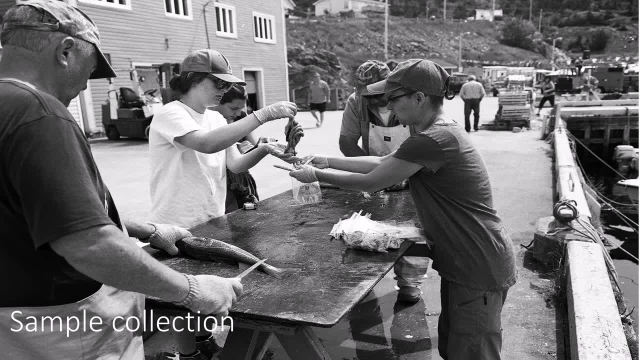 And what usually happens is a lot of Newfoundlanders go out, catch a lot of fish and then stock their freezers. Now because we're worried about plastic ingestion in fish, particularly codfish, which is what Newfoundlanders eat and catch. 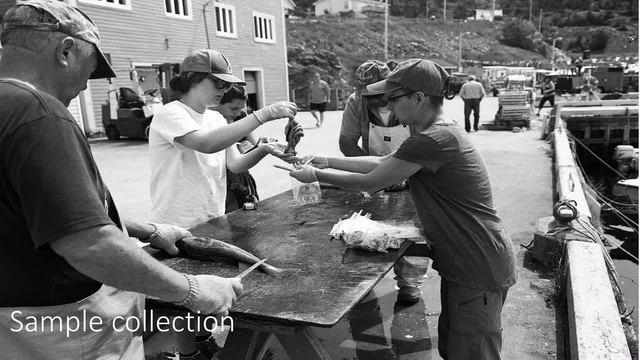 we go to the wharfs and we collect the guts from these fish. Now, most scientific studies sample fish from the water, from the ocean. We sample them from the human food web, So all of the plastics that we look at in cod. 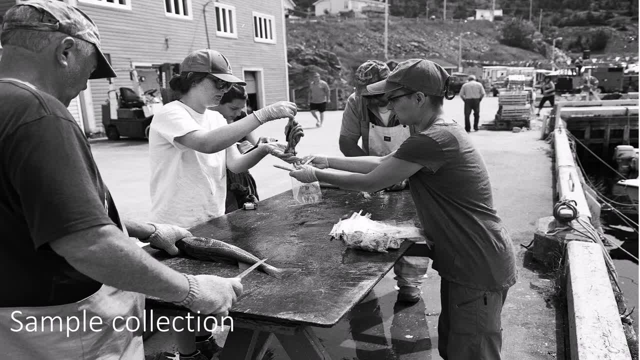 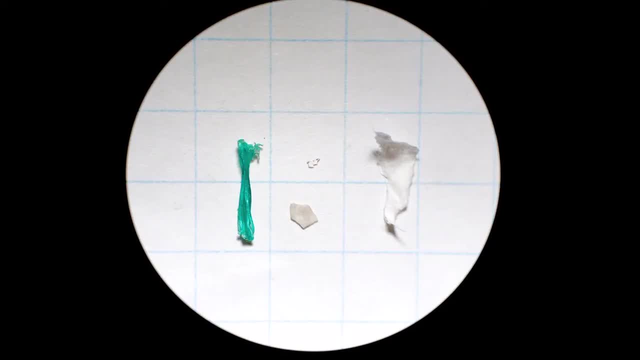 those cod were definitely eaten by humans. So this is another justice issue. Instead of sampling the ocean, we sample the food web. Now, the first time I found plastics two years ago, I was super excited because I'm a plastic geek and you find the thing that you study. 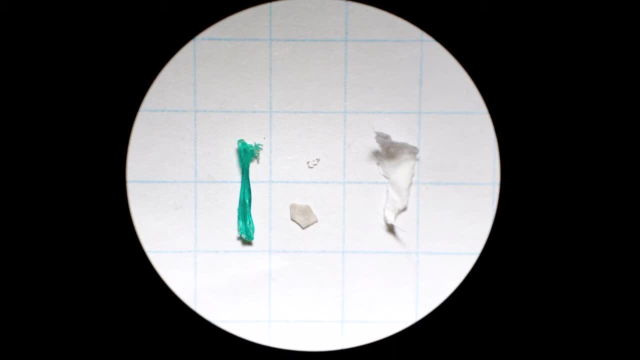 and it's really exciting. But then I realized that I had found plastics in cod in Newfoundland- Cod in Newfoundland. I cannot overstate how important they are. It's a major part of the various cultures that are here. It's a major part of sustenance and it's a major part of livelihoods. And in 1992, in Newfoundland the cod fishery collapsed from overfishing, from industrial practices. It devastated the province. It was the largest job layoff in Canadian history. It was a capital period And Newfoundland is not a very populated area. 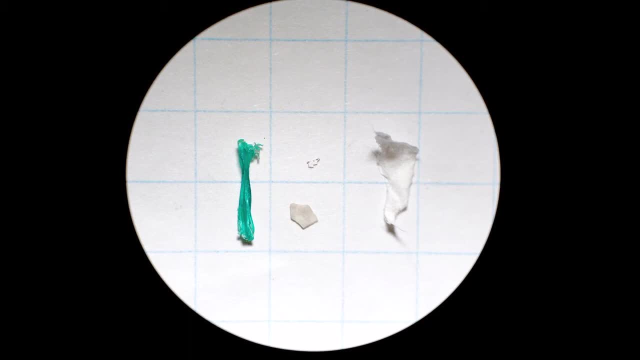 People still think and talk about the cod moratorium like it was yesterday, So I didn't want to add to that sort of harm. with my science I had just found out that cod in Newfoundland were contaminated. So this is the problem with scientific knowledge. 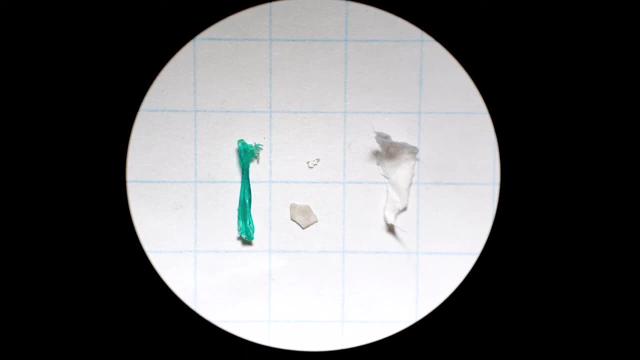 Even if you don't intend it to be, it can cause harm. It is not neutral, It's already part of these social economic networks. And if I were to just say, publish this out into the world and people found out that codfish in Newfoundland. 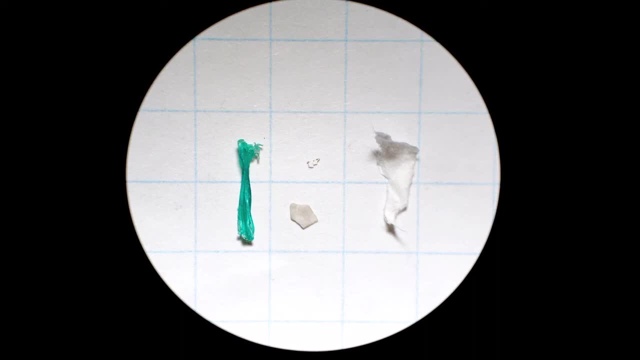 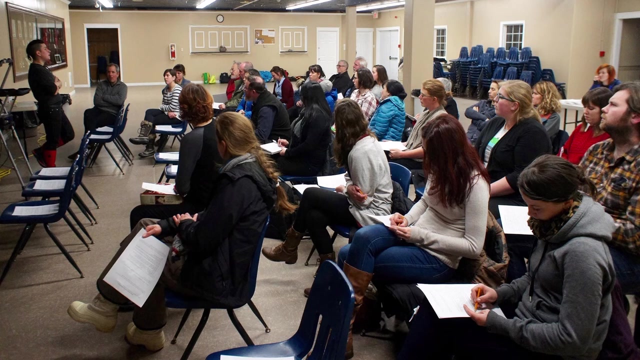 were contaminated that might have affected lives and livelihoods in a very negative way on a very grand scale. So what do I do? The answer is: I don't know. I don't know, but Newfoundlanders know. So I called a public meeting from the place where we gathered most of the fish guts. 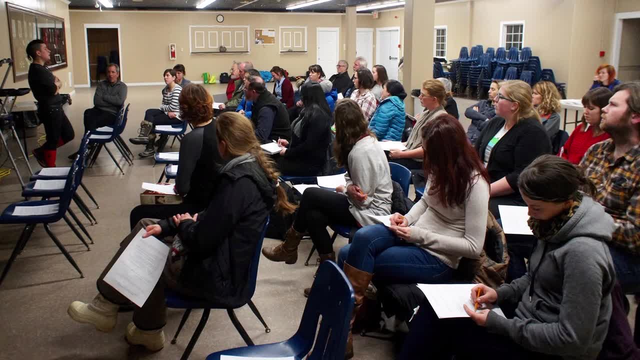 a small fishing community called Petty Harbour, and we asked them as a lab. this is what we did. this is what we found. how should we publish this? what can we do? This is now what we call community peer review. It is sort of like academic peer review. 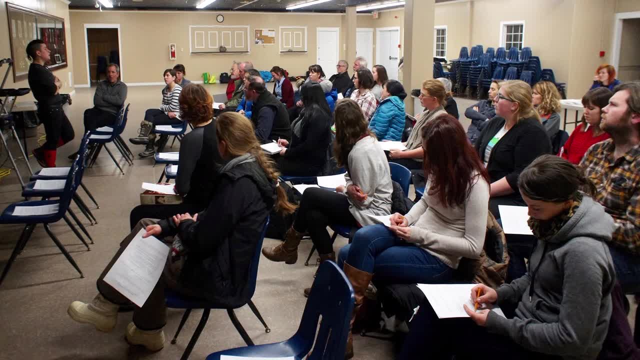 You ask how and why things can get published. but it comes out of a practice in anthropology. So anthropologists have long realized that sometimes they get knowledge that they shouldn't have or haven't earned: Sacred knowledge, very private knowledge, harmful knowledge, 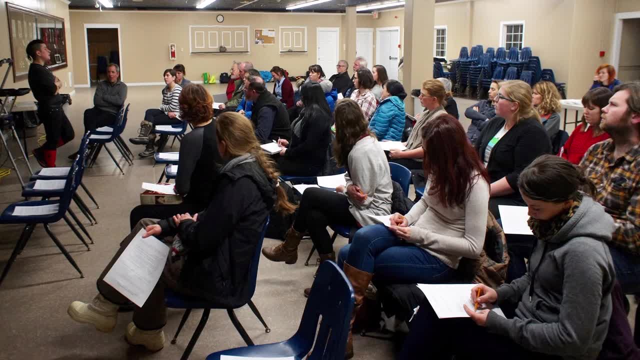 stuff like this, And so community peer review is a way for communities to determine how they are represented in science. how they are represented, It's about self-determination, it's about autonomy, and it's about giving citizens a place in science where they normally don't have one. 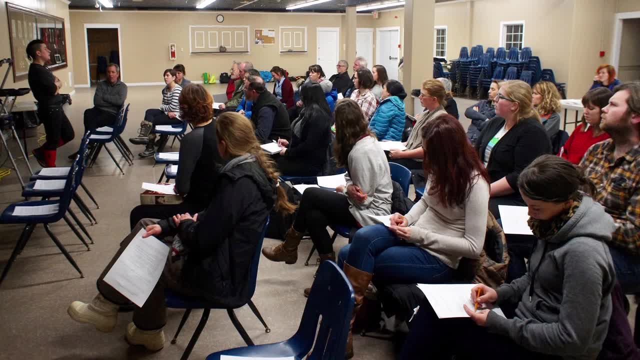 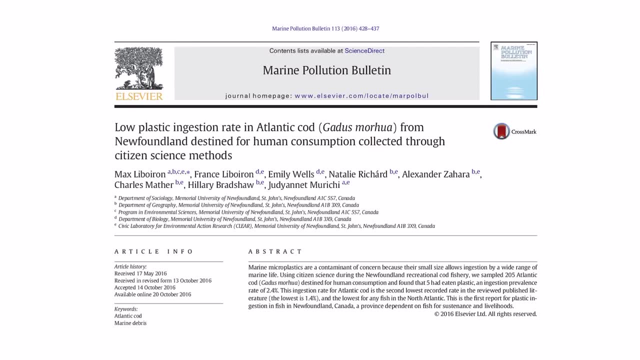 When I say citizens, I mean of a place, not of a nation, the people who are most affected by this. In our case, it turns out people said: please publish this. this is our first publication on plastic ingestion in cod, And that's because we found one of the lowest ingestion rates of cod in the world. 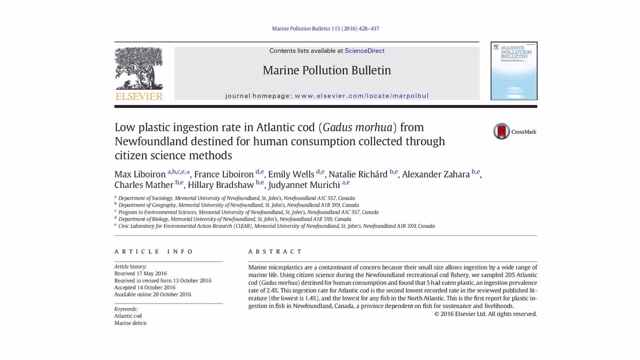 So because it was lower than Iceland and Norwegian ingestion rates, people said: please publish that, that's a competitive advantage. I said hey, it's still contamination. They said: we don't care, we're fishermen. I said okay. 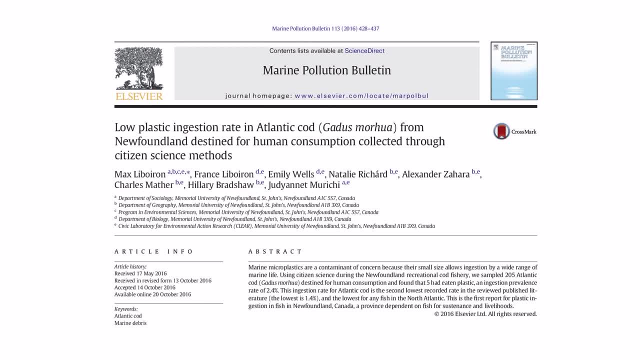 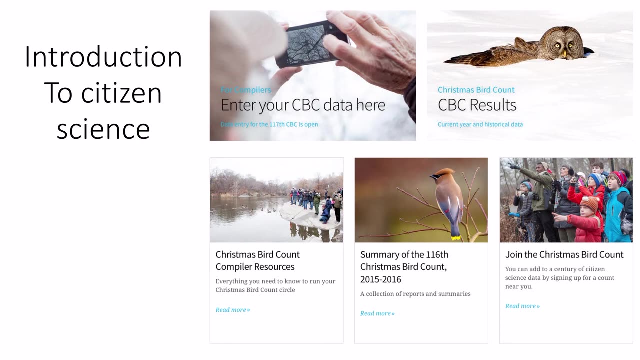 We do this every time. Every time we do an ingestion study, we then go to the community we got the ingestion samples from and we talk about the data and how it should be represented. This radically transforms how citizen science is done. Most citizen science is based on what's called 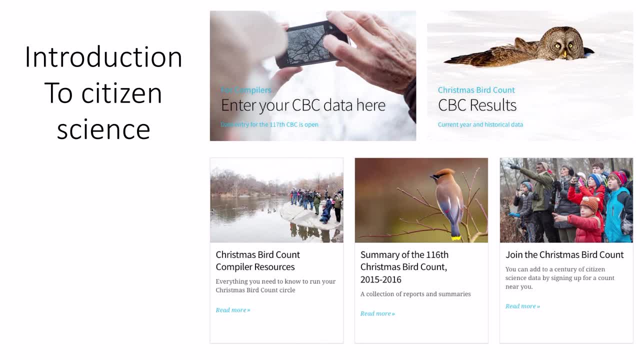 crowdsourcing and distributed intelligence. Crowdsourcing means using people- non-scientists- as sensors. The Audubon bird count is super famous for this. On Christmas, everyone goes out and counts birds, puts it in an app- very long-running population study. 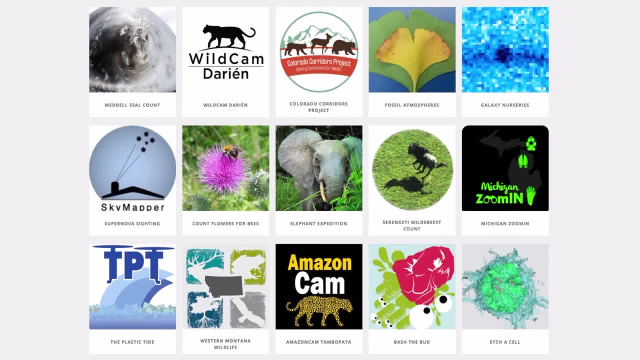 Zooniverse is another example of crowdsourcing. It's basically the Mechanical Turk of science. Everyone does a little bit of piecework. You count seals in photos, You look for blotches on photographs. Basically, you work for free for science. 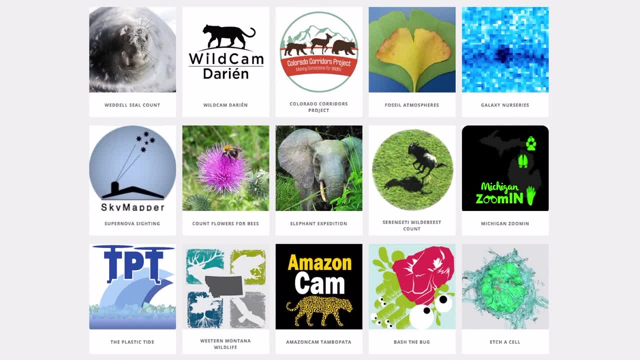 Of course you enjoy it, but it doesn't get to everyone. It's an equity. It doesn't change how science is done. It doesn't change who is likely to be doing this. It doesn't change the type of questions, type of science, type of knowledge that circulates. 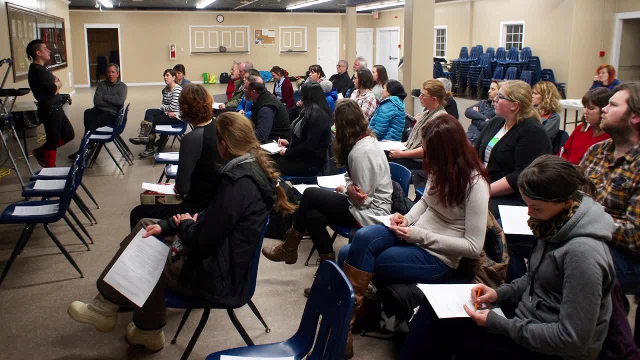 This is why we do a very different kind of citizen science, where we work more collaboratively and we work more as partners. We work for people instead of using people to work for us. The other thing we now do is those little papers that everyone has in their hand at this community meeting. 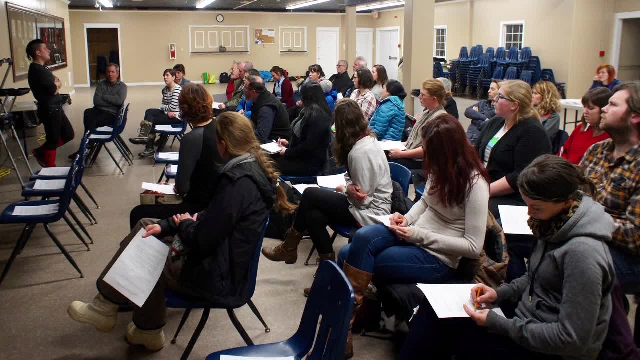 are surveys about the type of work we are doing and what they think is most important, and the type of research questions that we aren't asking. Since these have started, we have not done as many surface trawl studies or shoreline studies. Instead, we look almost exclusively at ingestion studies. 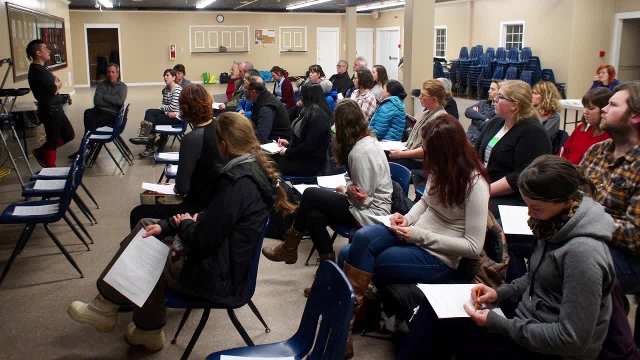 because that's what people in Newfoundland are concerned about. It's a very different way of doing citizen science. that's justice, participation and collaborative- as opposed to using people as what we call data bitches- free labor, even though they want to, for science. 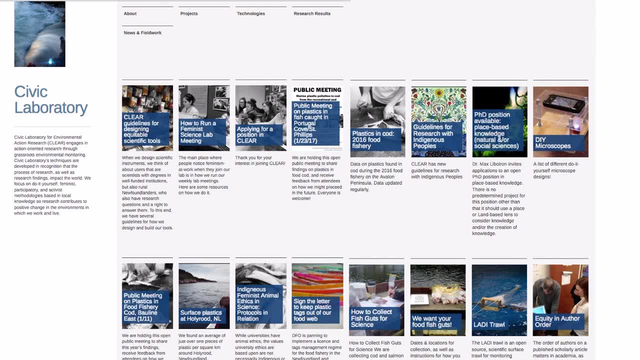 Thank you very much for your time Again. my name is Dr Max Lebrun. I'm the director of Civic Laboratory for Environmental Action Research. If you have any questions, you can look at our website online at civiclaboratorynl.